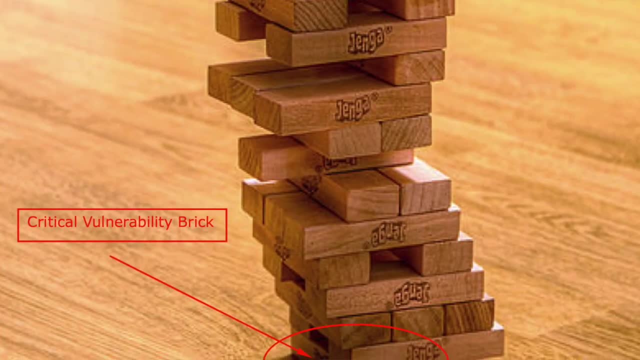 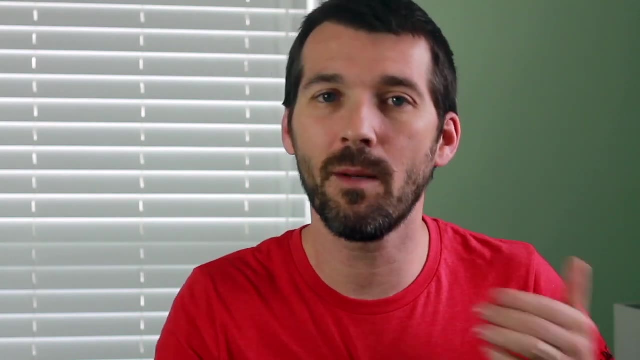 thing, And the whole point of doing a risk assessment, is finding where the vulnerabilities are, the weaknesses, categorizing them So you understand how bad the risks are, and then coming up with remediations or things that you can do to fix the vulnerabilities. 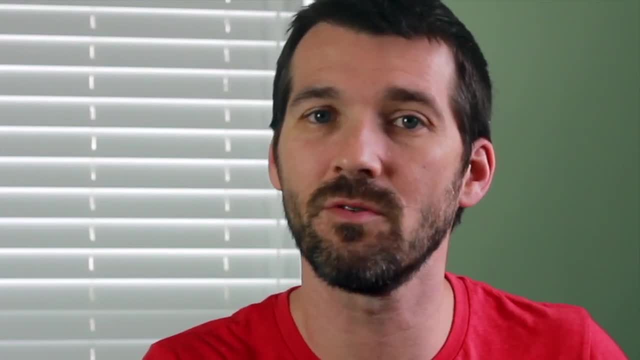 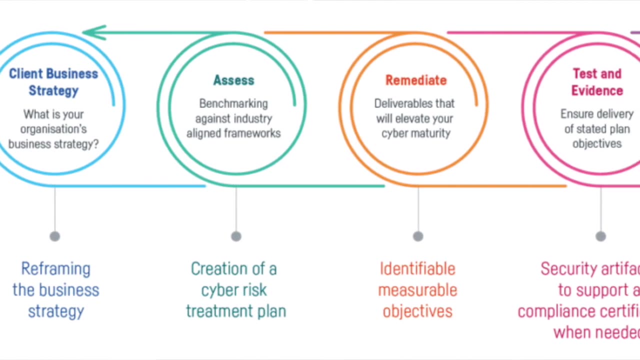 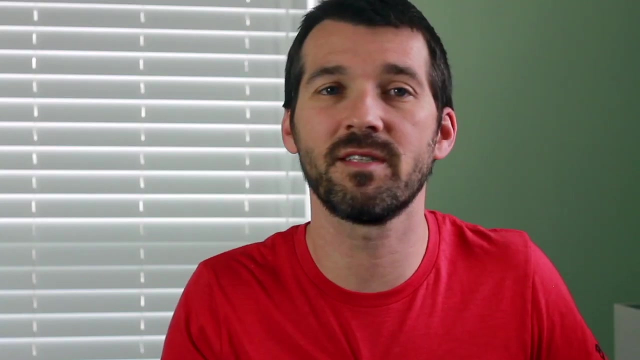 or just to reduce the level of impact that those vulnerabilities present if they were exploited. It's very important. It's an ongoing function within the cybersecurity kind of office or the information security office, And in this video I've done risk assessments for years right, And I've gotten some requests. 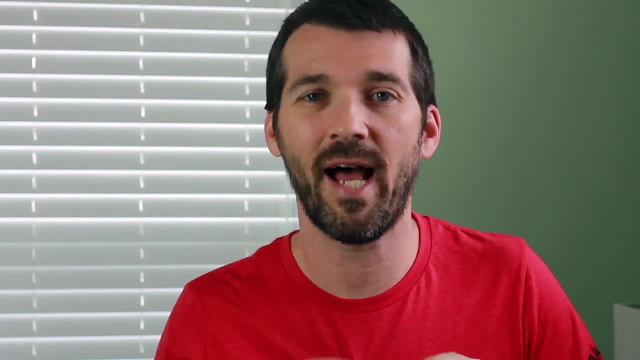 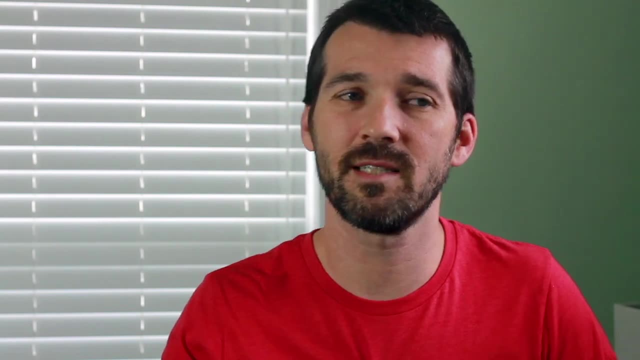 from the community. Thank you for providing those requests on how to do this. I'm just going to shoot from the hip and tell you exactly what you need to know in order to execute a risk assessment. I'll be focusing on information system, because that's more of the commonwealth. 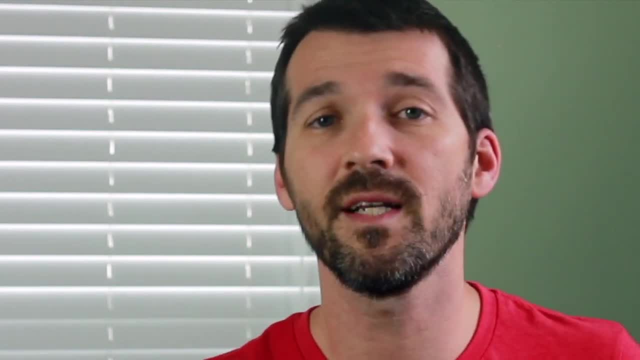 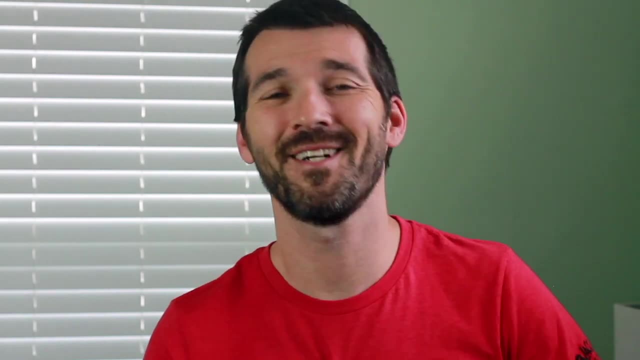 Let me introduce myself If you're new here. my name is Jerry Ogier. This is Simply Cyber. It's a YouTube channel designed to help you make and take a cybersecurity career further faster, and on this channel we do all sorts of stuff: how to get into cyber with no experience. 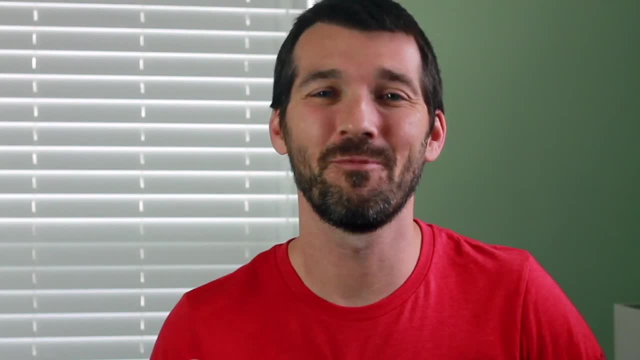 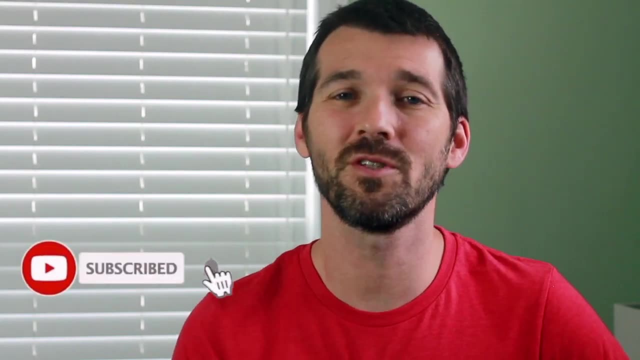 how to set up a pen testing lab and how to do risk assessments- giving that GRC a little love. So that's what we're doing today. If that sounds interesting to you, scroll down, hit subscribe. We push videos at least every Monday. Sometimes we do live streams, kind. 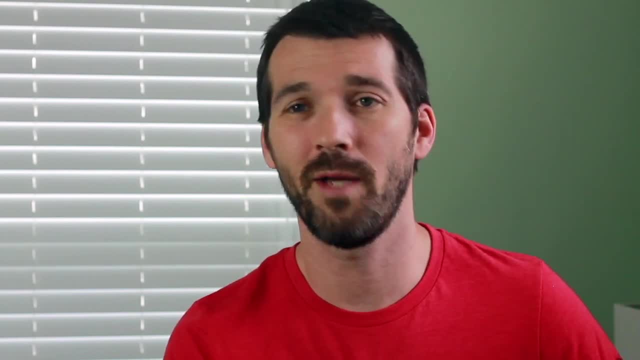 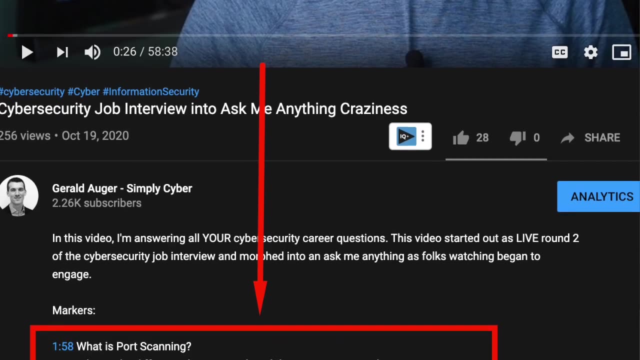 of renegade style. So stay tuned. If you hit the bell for notifications, you'll be made aware when we go live. So check it out. Anyways, use the time markers below to jump around the video, or if you come back and you want to get clarity on some particular part, that's what. 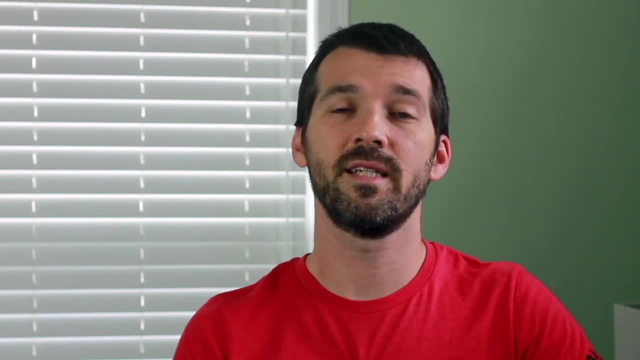 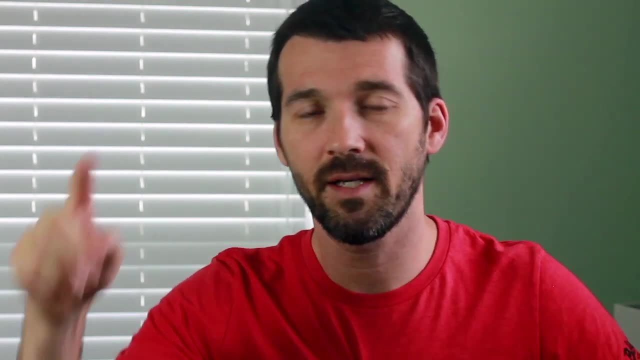 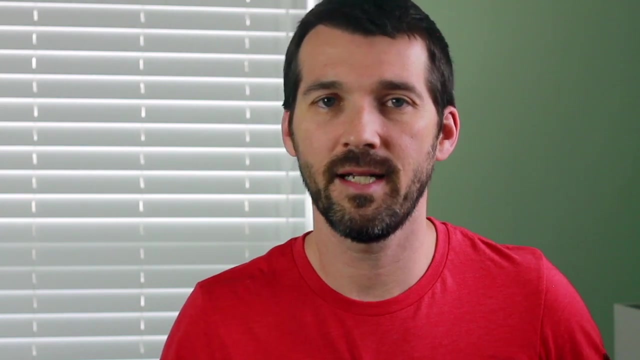 they're there for as a convenience to you. So let's dig into it. Okay, so the risk assessment: it's a pretty standard workflow and you would want to go back to the beginning with some iteration, either annually or triannually, depending on how large a system it is that you're doing. 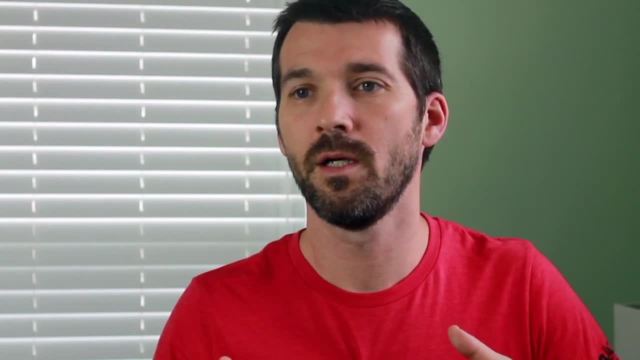 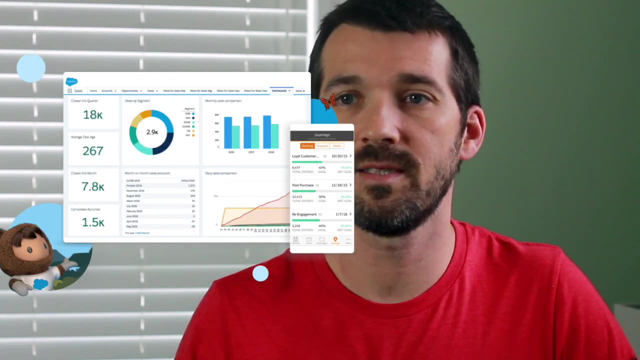 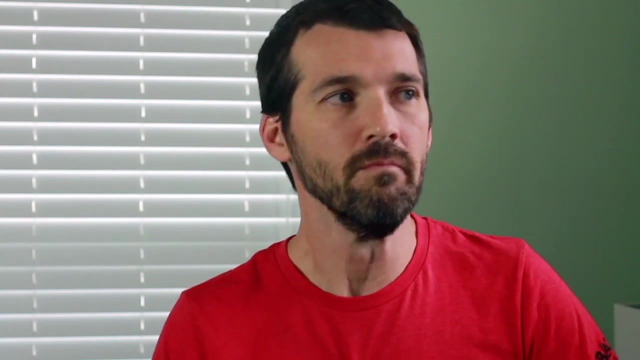 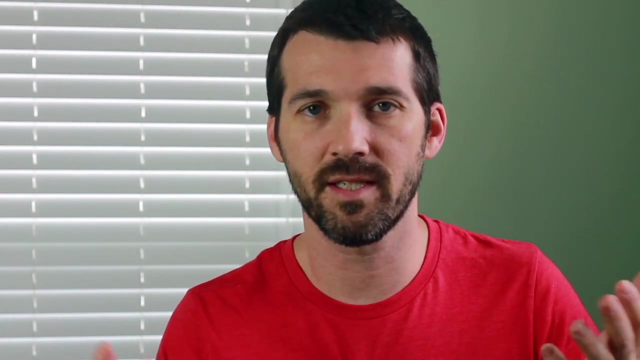 But basically let's just take a simple solution. like your organization, you want to start using Salesforce, right? Salesforce is like a CRM type tool for tracking contacts and stuff like that. Okay, so what is the risk to your organization to start to use that platform? right? This is just an example I'm making up on the fly. Well, 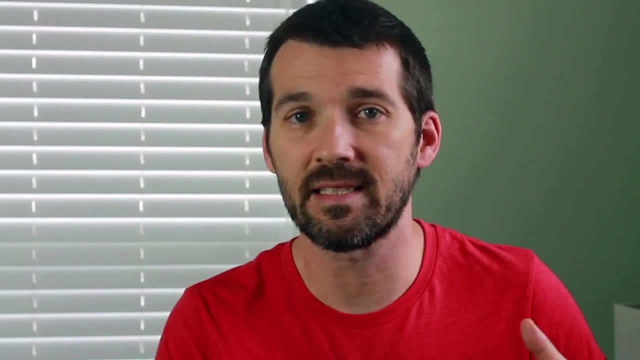 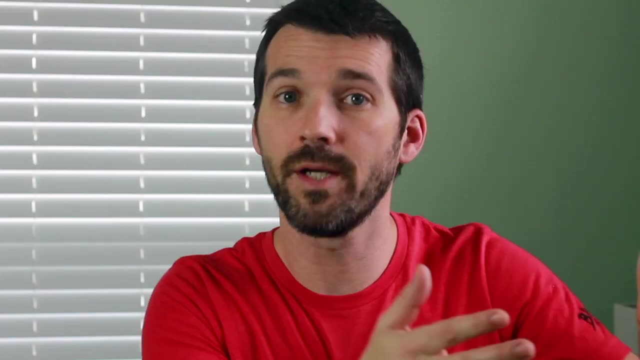 first you got to understand how are we going to use it. What is this system like? So you've got to do data gathering, okay? So because it's cloud based system, we're going to reach out to the vendor right Salesforce and get as much information as we can on it. What is the 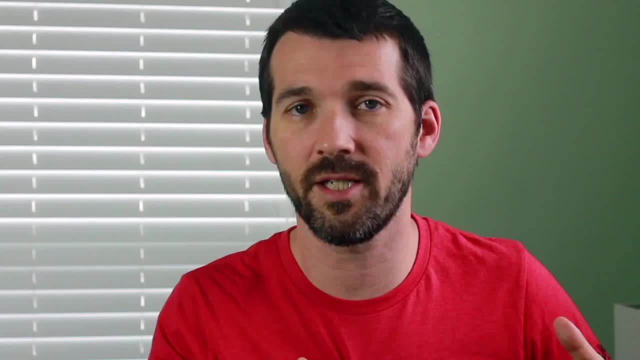 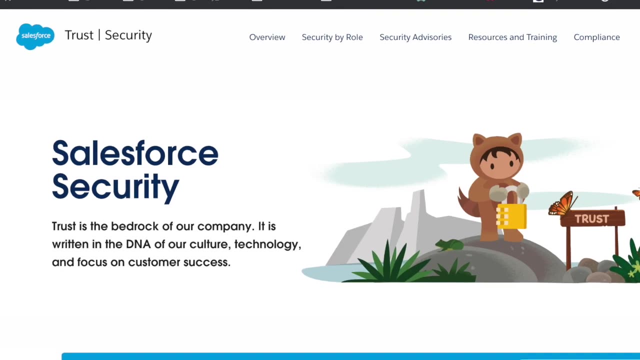 tech stack. look like. What is Salesforce like as an organization? What are you guys doing? Do you subscribe to cybersecurity framework? What level are you? Do you get SOC type two audits? Can you provide a recent pen test? right, If it's cloud based system, you're going to want them to have. 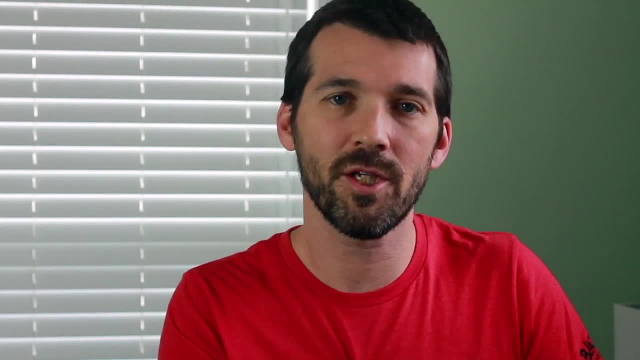 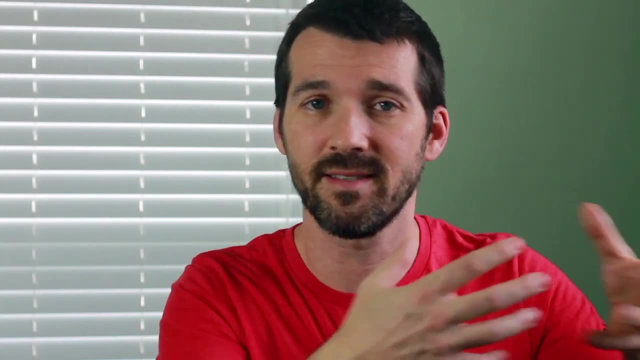 some pen testing done right, So you get as much information on the solution and the company as possible. Think of that as just like data Intake for like, or it's Intel right, It's intelligence on how you can do something. 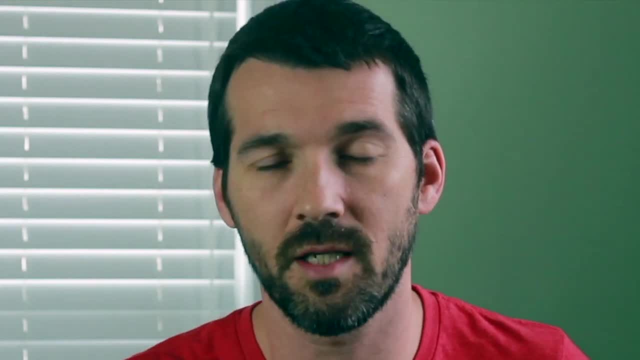 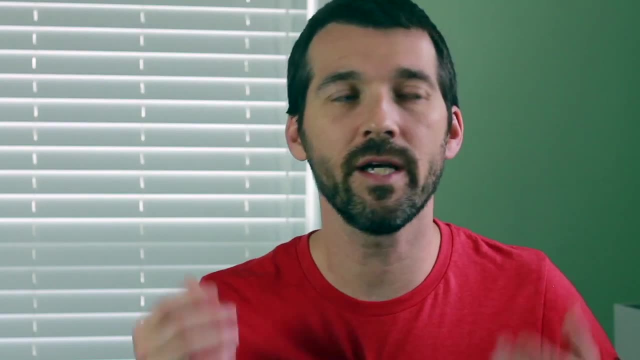 Secondly, we want to pivot. If you think about it, our organization is going to be using it. How are we going to be using it? Who is going to be using it? Again, it's all about Intel. You cannot do risk analysis without intelligence Like you. just what are you basing your risk? 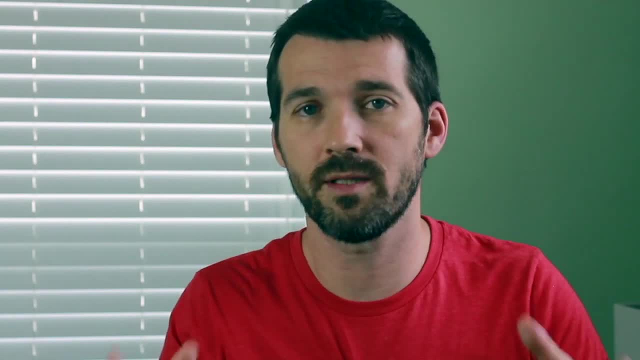 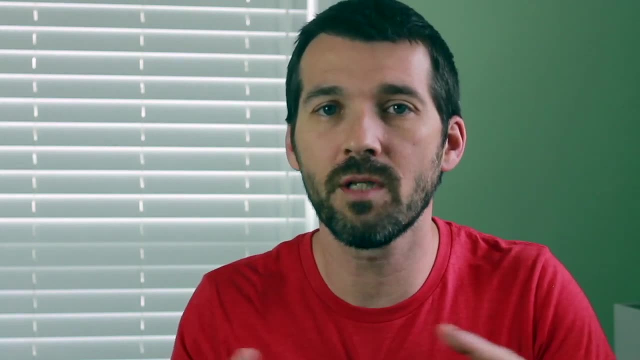 qualification on Right. So okay. Who wants to like? who's requesting this? Like, okay, So the CEO, All right. So this is going to be okay, CEO. who's going to be using this? This is just the marketing department. Is it the entire company? 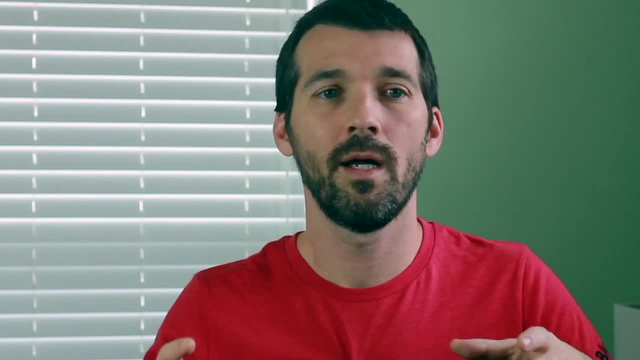 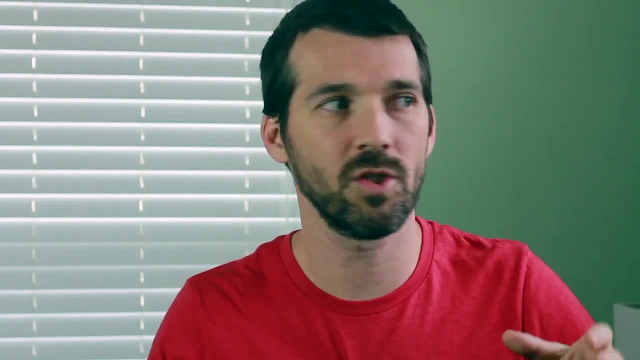 Are there third-party vendors involved? Okay, So, once you understand what is the use case and- and try to exhaust all the use cases right Cause sometimes you'll get a solution- You'll do your risk analysis on it And there's additional functionality that they didn't even. 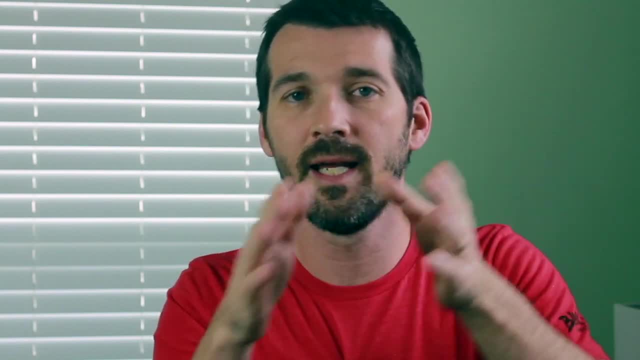 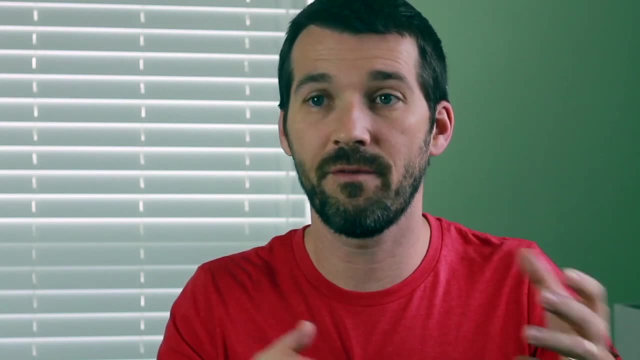 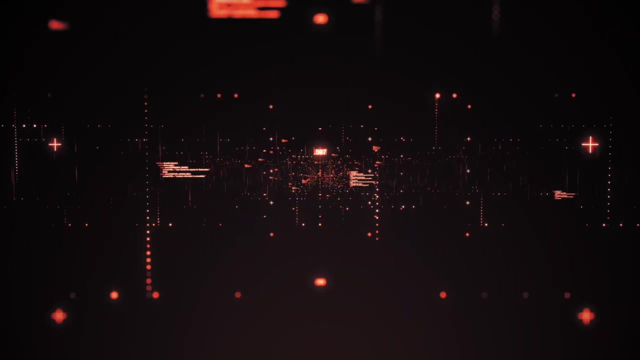 know about that, They'll start using. This is why we come back cyclically and look at the products or the enterprise, or In order to assess and understand, um, if the risk has changed. Okay, So now that we've got our use cases and we've got our tech stack, what kind of data's going in there, Is it? 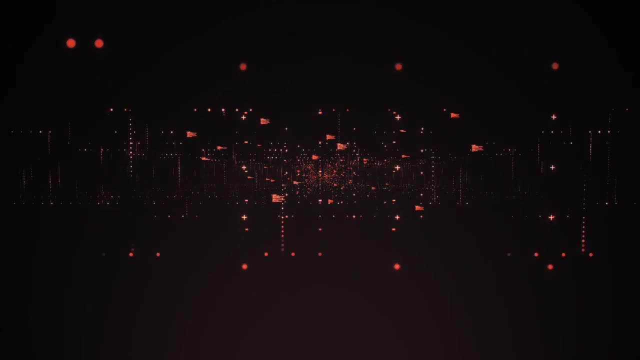 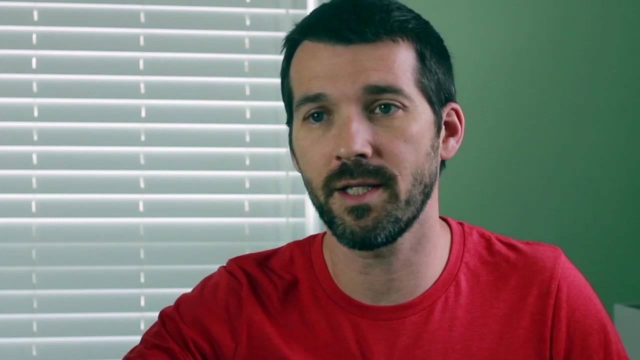 just: is it fake data so we can do simulations? Is it actually our customer client data? Is it data that we have procured from some third party that we've agreed to protect in some way? Right, So the government gives data all the time And there's certain restrictions around how you handle it. 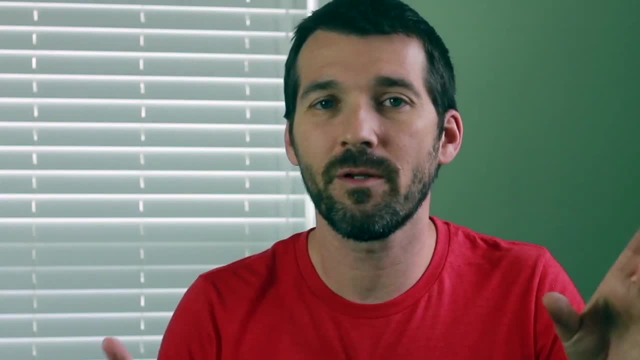 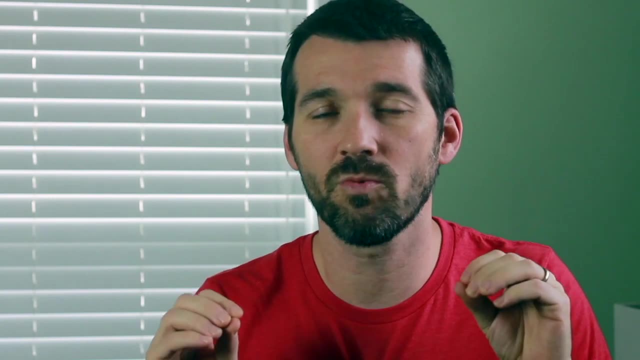 What is the data? right, I know that Sony is the kind of company that, yeah, they do the work. but, right, I know we call it cybersecurity. but think for a minute, people, it's called information security. right, Cyber is just a way sexier term to throw around, but like information security is. 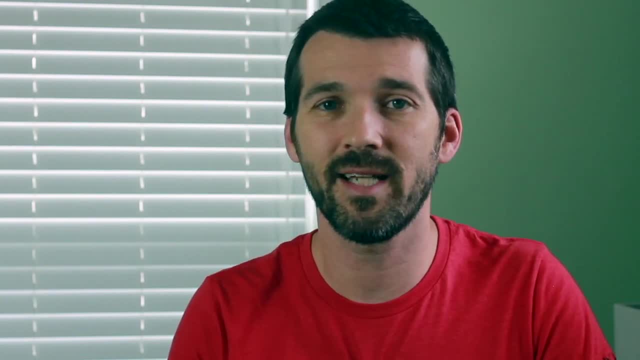 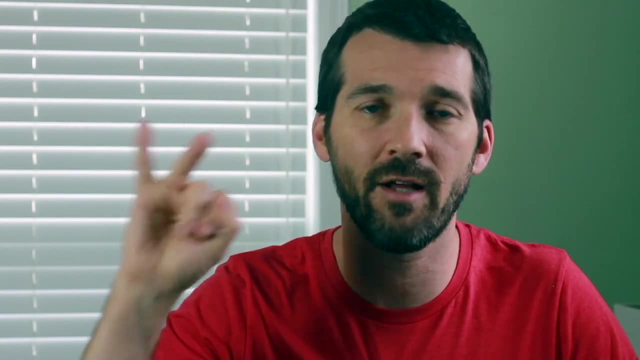 what we're doing. We are securing information. So, at the end of the day, the systems are important to protect, So they're available to the user base, but the information is what I am concerned with. The confidentiality, integrity and availability of that information is what I'm. 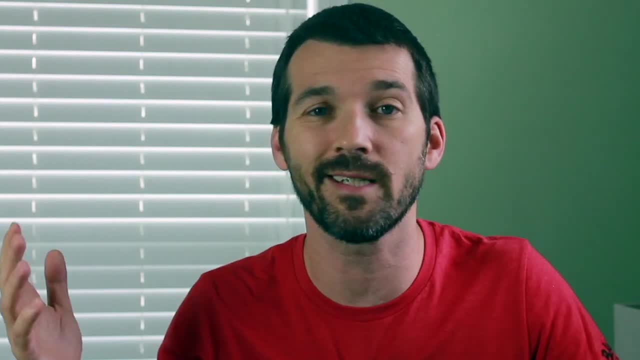 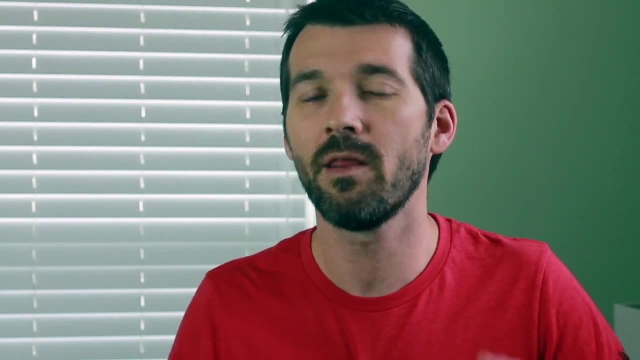 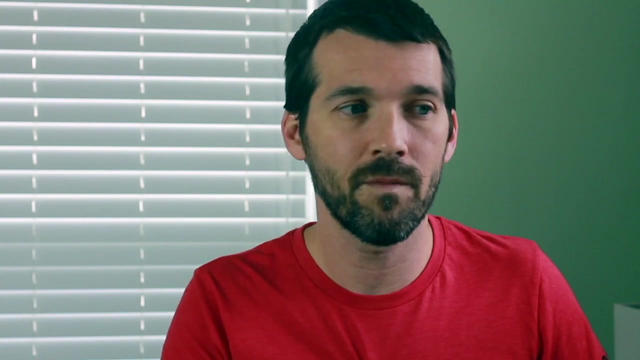 protecting. So I need to know: what information is it right? Is it like super secret patents? Is it the Coca-Cola formula or is it just public source marketing material right? The level of control that I need to invest in, both from a financial contribution and a resource perspective changes. 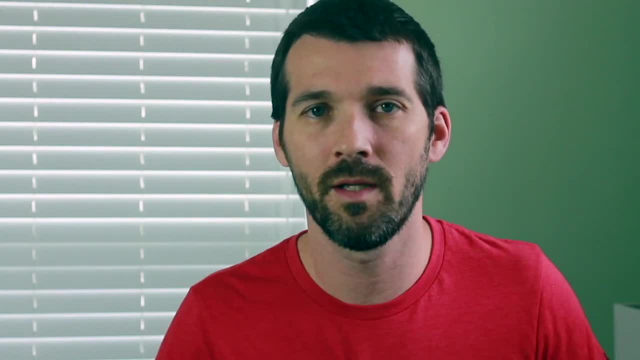 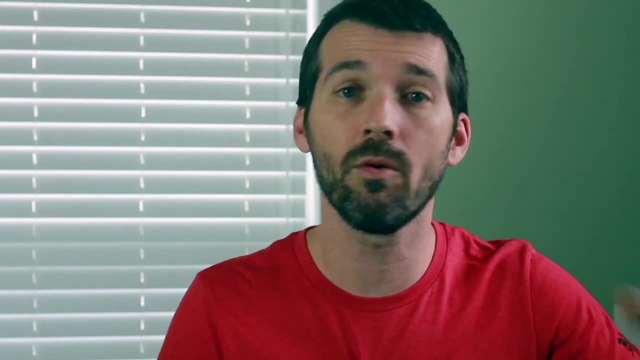 if the data is less important, right, I don't need to put as much control in. The impact is going to be less Okay. So once you get all that information, you begin to analyze: okay, how do people authenticate to this thing, How do they get access to the system, How is the data brought in? and 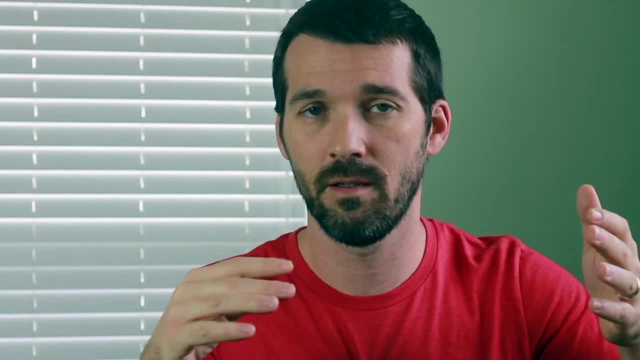 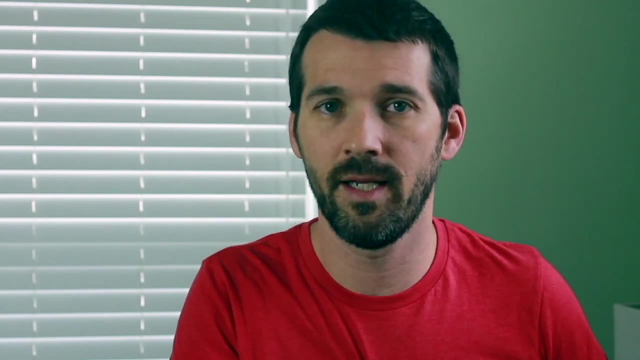 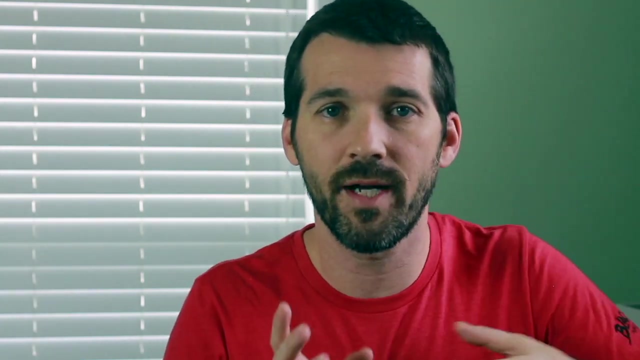 brought out. Is the network traffic encrypted? Is Salesforce required to protect our information? Do they have data at rest? Have they had a breach recently? If we decide to switch from Salesforce to whatever Oracle, whatever, can we get our data out of there and moved into something else? 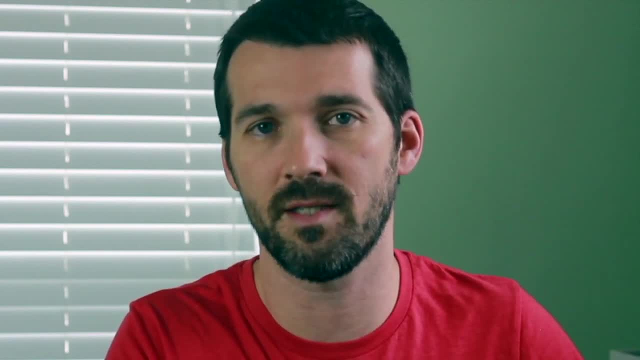 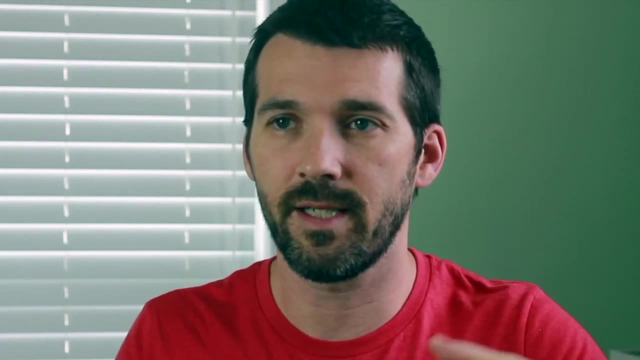 right. Think holistically about the life cycle of the use of the system: getting data in, using the data, who has access, who doesn't, and if there's an incident, how that's handled. Then when you want to terminate the relationship, okay. This is bigger than just tech, right? This is 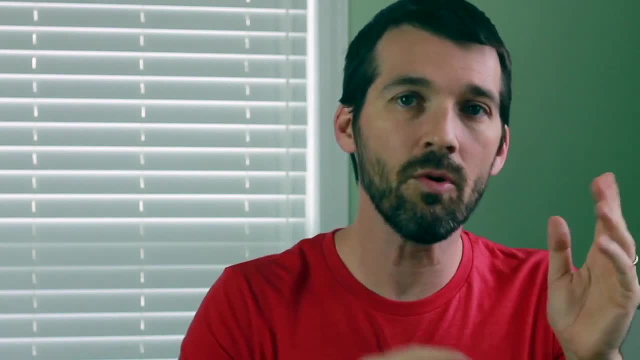 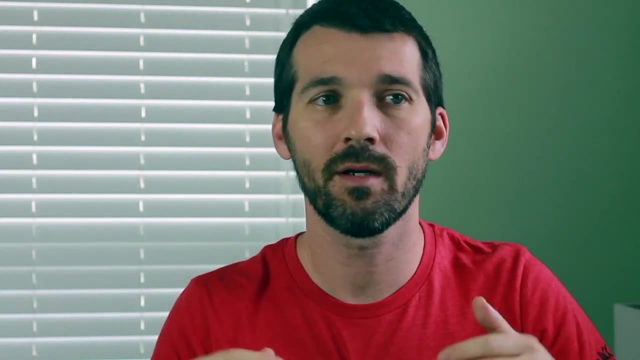 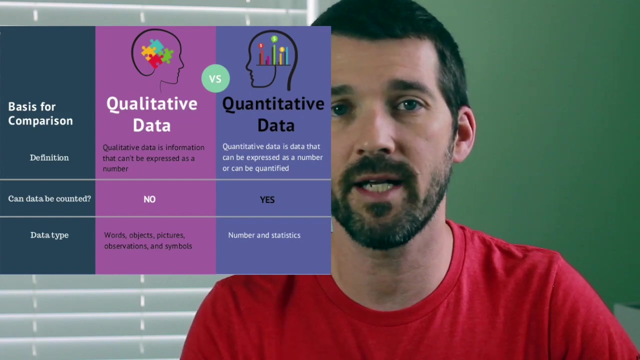 bigger than tech, but there is tech pieces to it. So once you've gotten the whole picture now, now you are prepared to do really the risk qualification. There's different ways to do it. This is a qualified risk assessment technique. There is a semi-quantitative risk assessment. 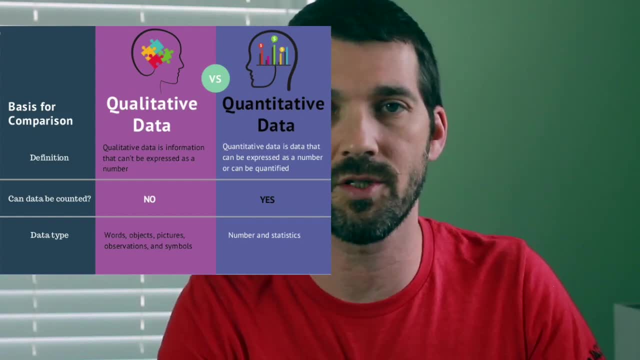 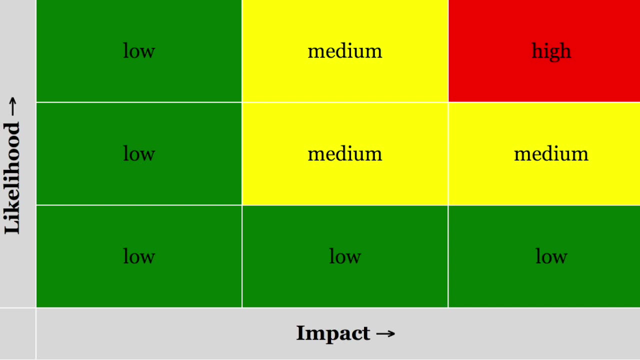 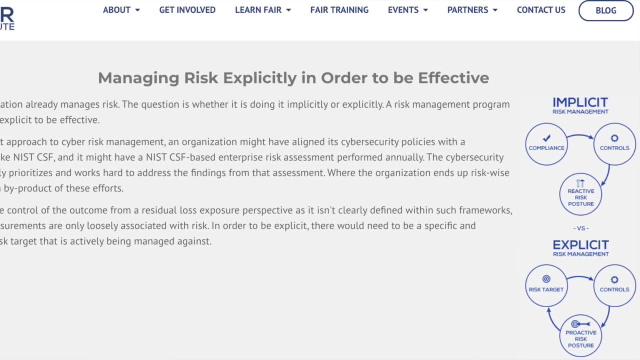 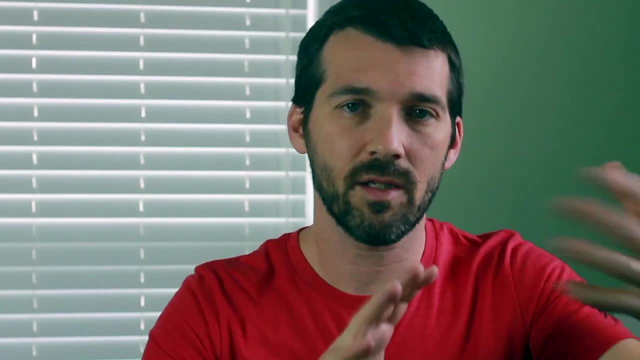 FAIR F-A-I-R risk assessment, which is more of a semi-quantitative risk assessment technique using probabilities. It's actually quite good, so I recommend you look into that. But once you've got the whole picture, then look at where the weaknesses are. 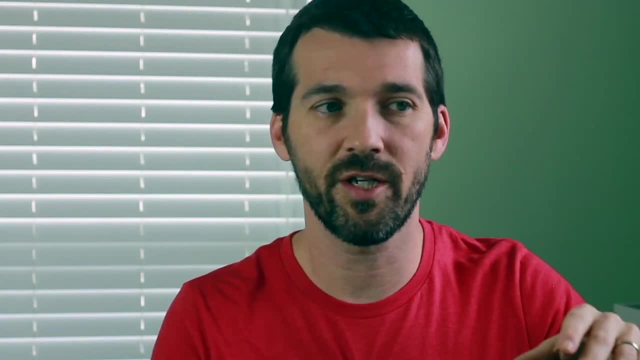 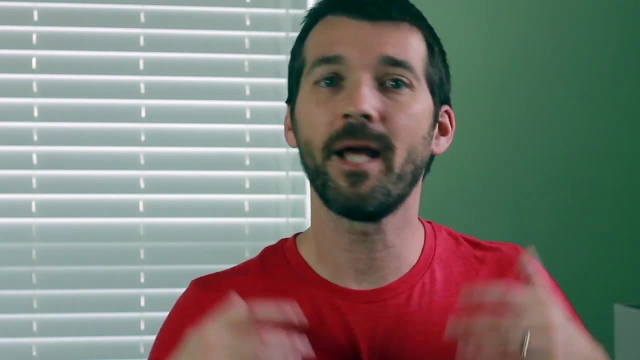 Okay, so like they have a mobile app but it's kind of trashy, or they don't have multi-factor authentication capabilities or they don't support federated authentication, or they don't have data at rest encryption. Okay, now some of the controls and some of the 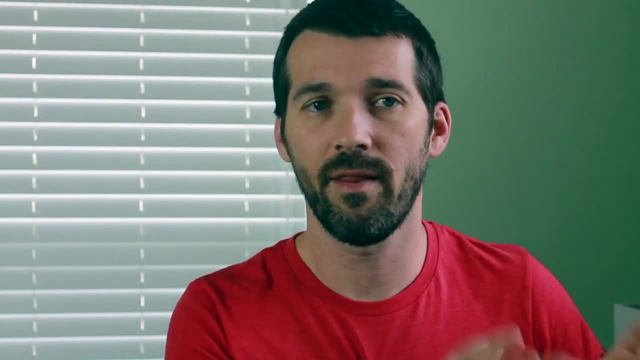 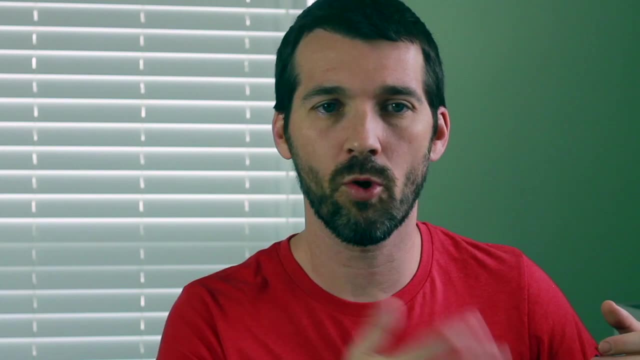 weaknesses that are on the cloud side. you're not going to be able to do with that. You'd have to use other. like you can't introduce security controls, You would have to do working into a contractor or whatever. There's mechanisms around that. but identify all your weaknesses right. 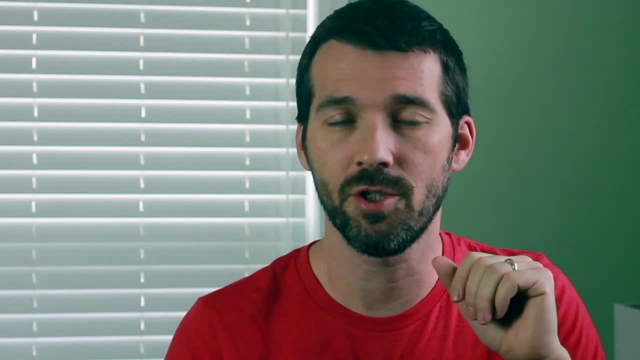 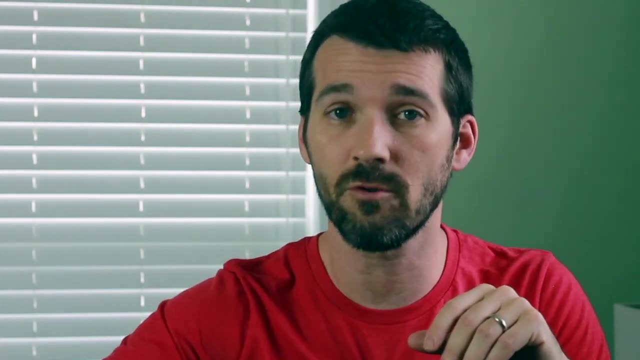 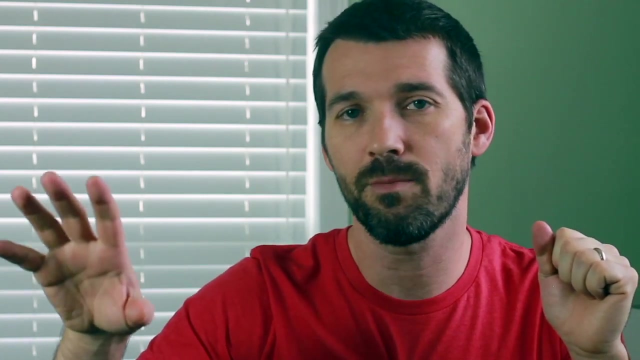 So let's just say that they don't support federated authentication as an example, which means you can't use your organization's username and password to authenticate to the Salesforce platform. Again, this is just a made-up example. I don't know about Salesforce. They probably do have federated authentication support, So that means: 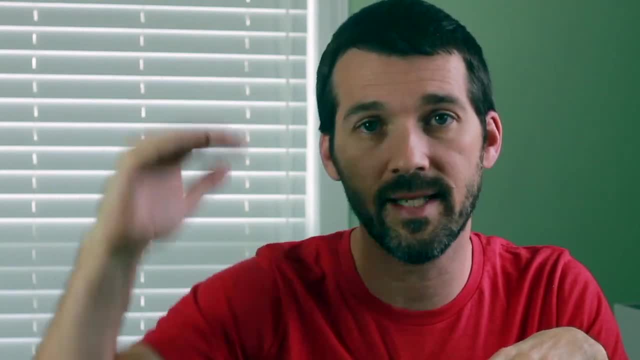 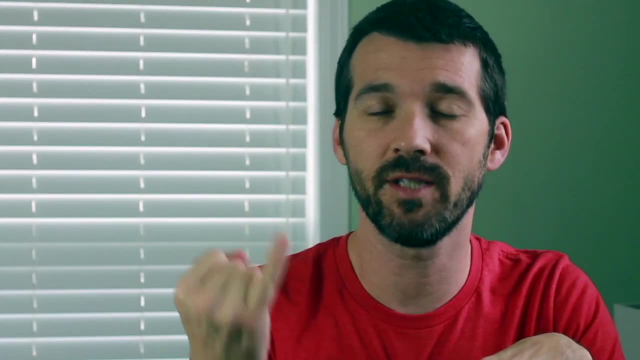 that someone has to create local accounts at the Salesforce cloud platform and all your users are going to log into that. Okay, so what does that mean? First of all, that means someone has to manage the accounts, right. So everybody that wants a Salesforce account- someone on your end. 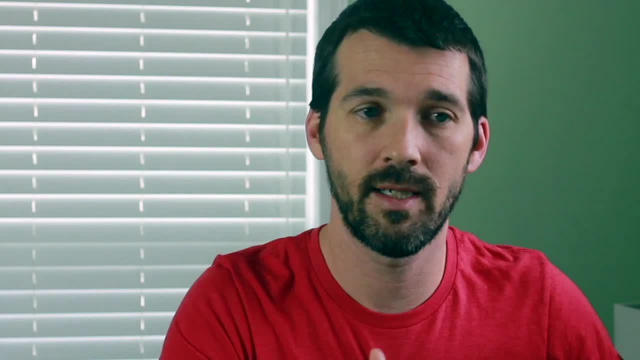 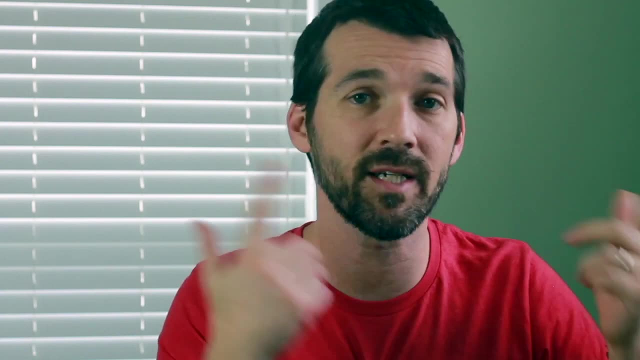 has to be the administrator to go in and create accounts right. So that's a level of resource that needs to be considered. Secondly, you know, maybe Salesforce doesn't require strong passwords, so that would suck and it makes the password easy. 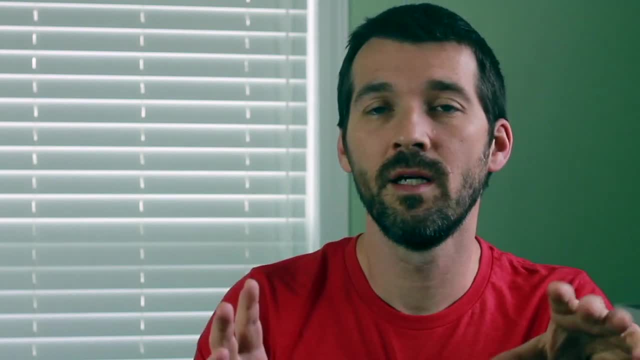 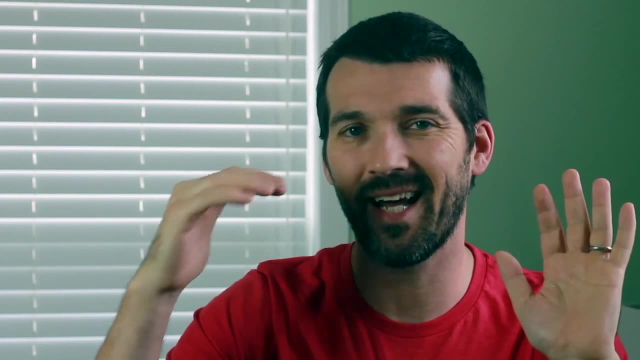 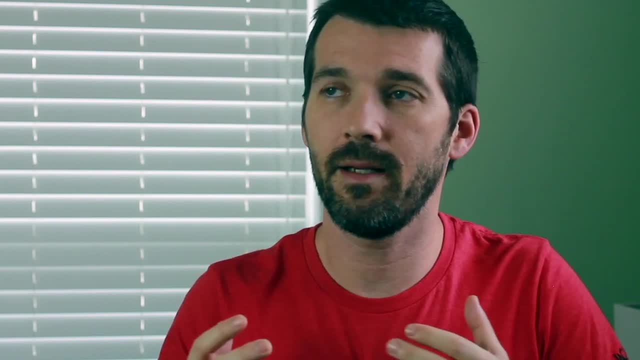 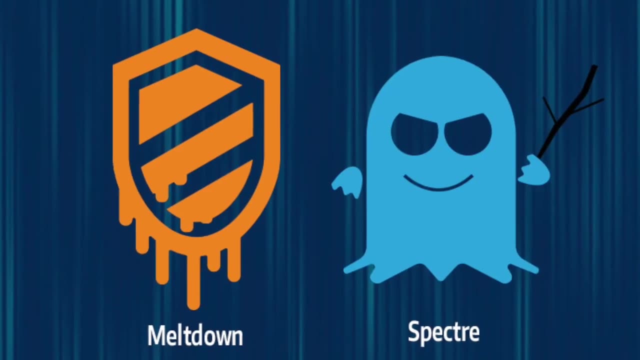 likelihood of this being exploited. right And an impact is: how bad is it when it does get exploited? To put it in perspective like the Spectre hardware vulnerability from a couple years ago, like yeah, that's really bad and there's been some proof of concepts and stuff. 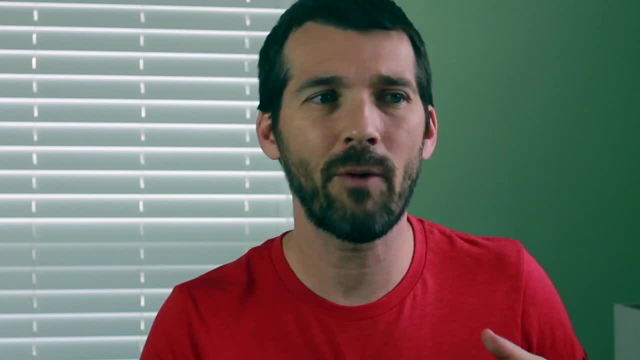 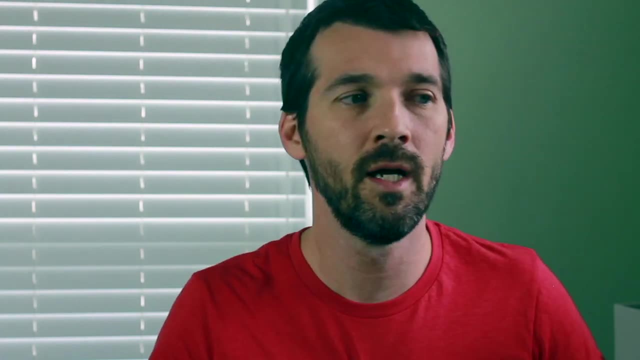 but like the likelihood is wicked low in my opinion and I wouldn't really put a lot of resources and effort around protecting and reducing the risk of a Spectre attack right, That's a low likelihood- Someone getting phished for their. 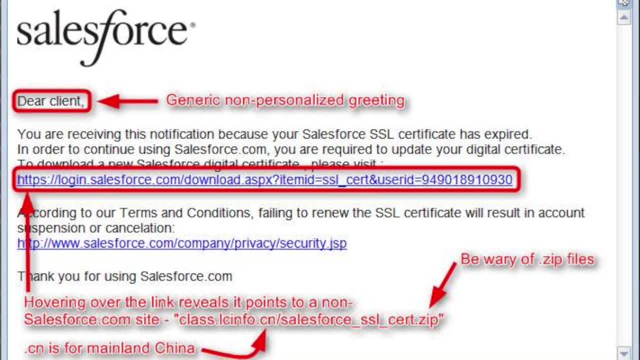 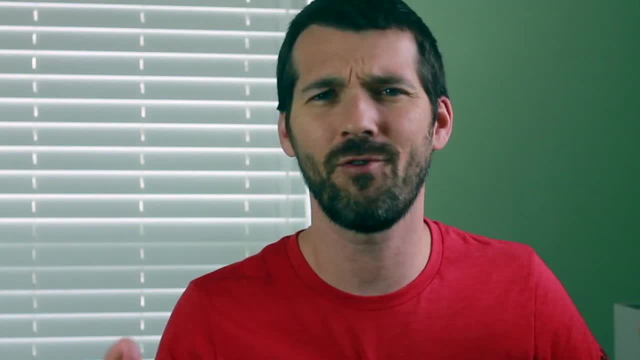 Salesforce credentials for a local account and someone getting into that, that's a pretty high- that's like medium to high likelihood, because phishing happens like all the time. like 20% of all attacks start with a phish right, So that's a bit higher. Now what is the impact of? 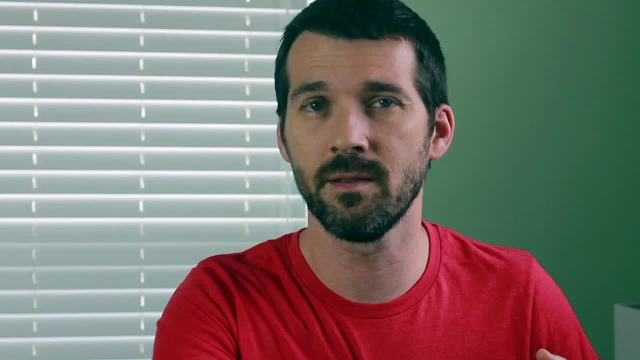 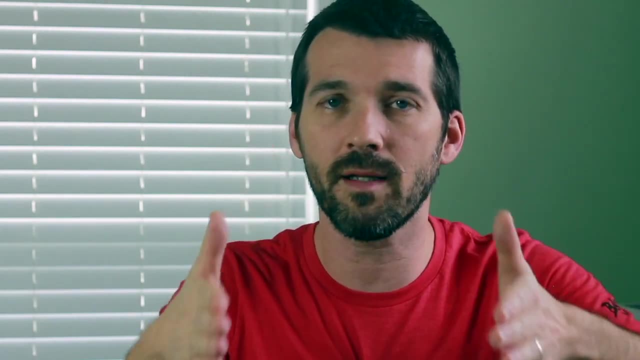 that Okay. so let's assume a threat actor phishes you and gets your creds. What does that mean? Well, the impact is that they get access to the Salesforce data. Now, if you've compartmentalized, who gets what data, access to what data in there, or the data is like: 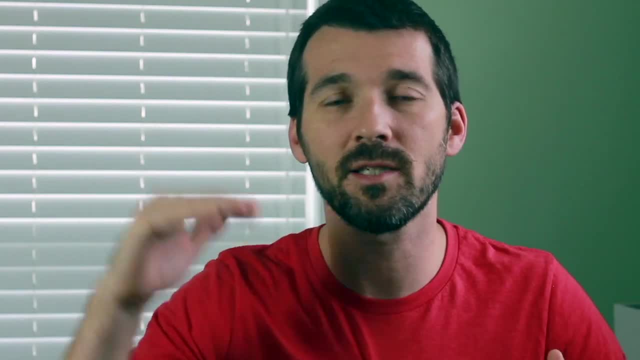 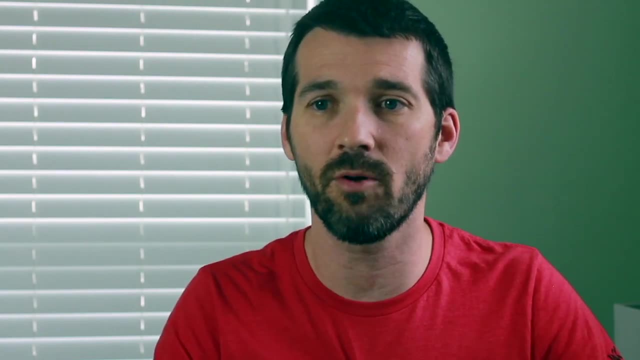 marketing material, not PII. well then, the impact is lower. right, It's not terrible if someone gets in there, because it's limited and Salesforce would notify us, or we have IP restrictions around where you can log in from, So if it comes from out of the country, it doesn't. 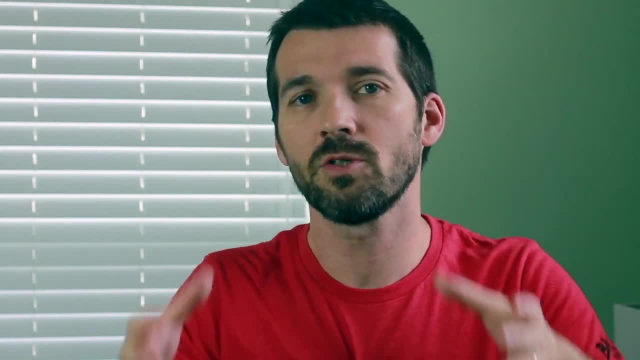 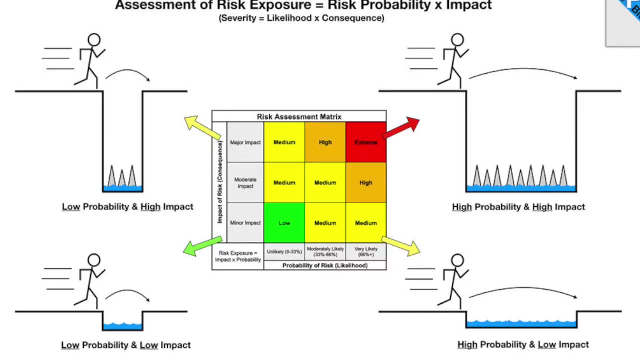 let you log in right away. right, For example, those are controls. So once you have your likelihood and your impact for all of your known vulnerabilities, then you start to say, okay, like, let's categorize these, Let's put all the bad ones up here, the medium ones here, the low. 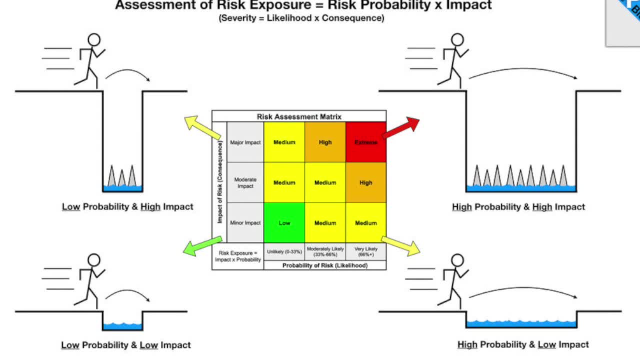 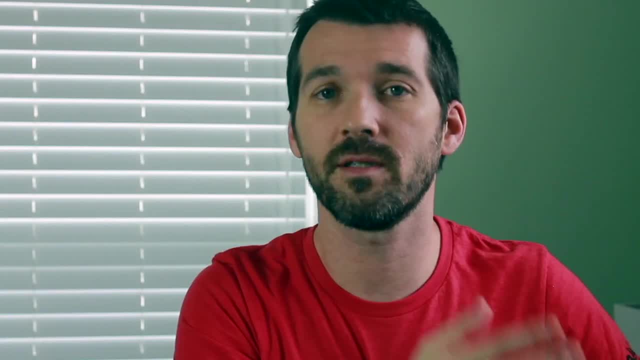 end ones here and then you present this to management. Hey, management, you want to go use this platform? These are really bad things that you absolutely need to do. Salesforce, in this example, doesn't support SAML authentication- federated authentication- and they need to. 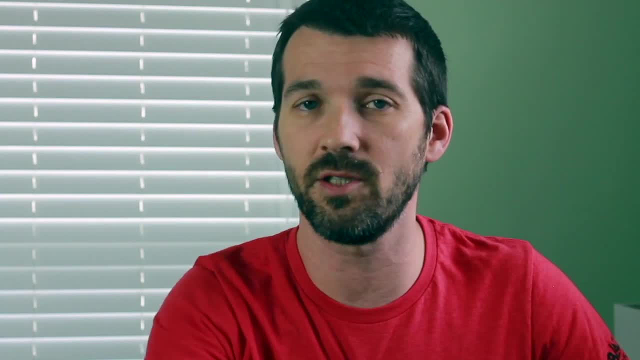 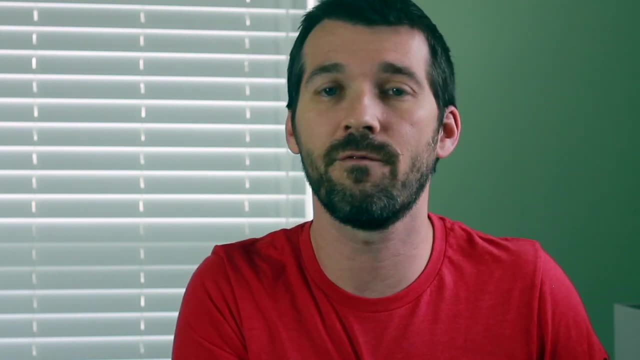 So before we do business with them- because it'll eliminate all those risks I just told you about- before we do business with them, they need to put this in. So then you can start turning the screws to the vendor and say: you guys need to put this in if we're going to do business together. 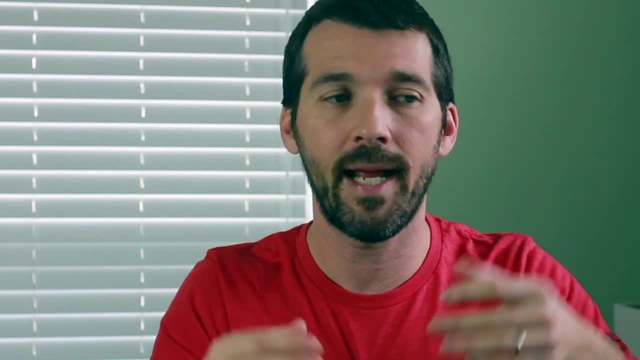 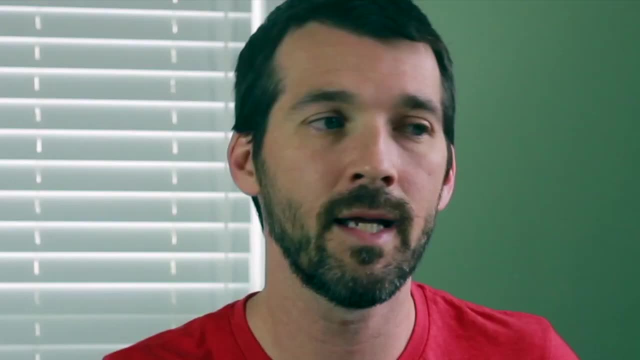 right, Or they offer either choice. and then you tell your organization: listen, you need to do federated authentication, We cannot use local accounts. The risk is too high. And now it gets into the culture of the organization. tone at the top how serious. 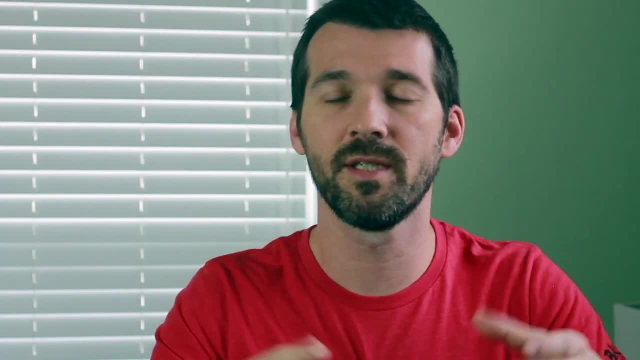 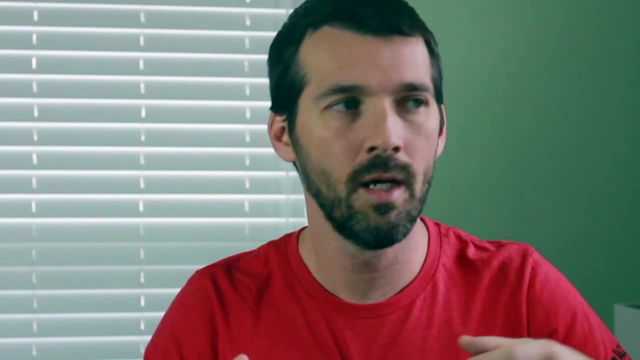 are they about cybersecurity? They put it in: the risk is reduced and you can go a little bit further. So you do that rinse and repeat A lot of times. people will accept the low risks because they're low, but you have that information And then you can come back a year later.